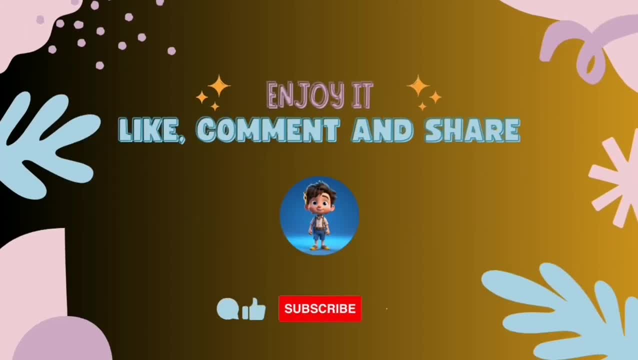 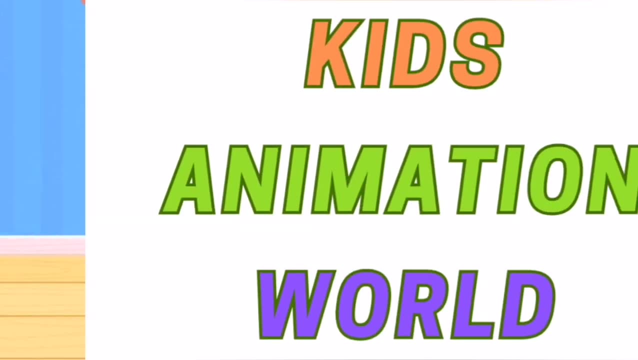 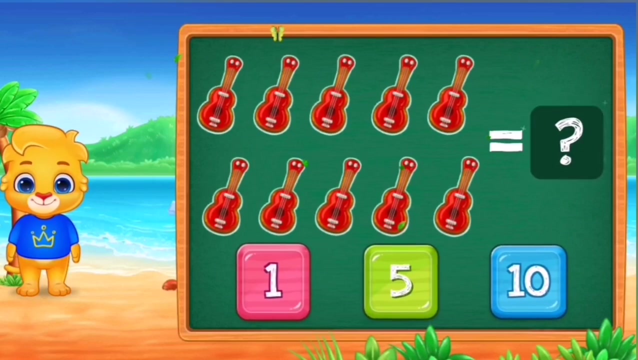 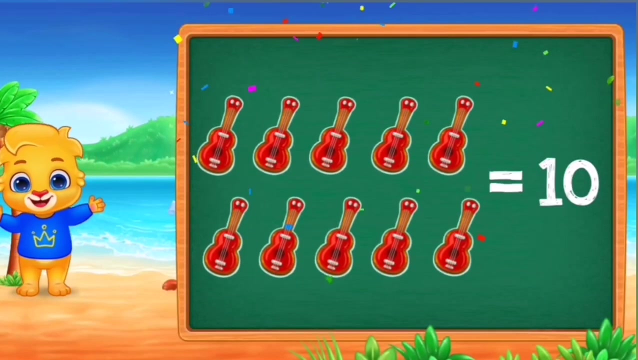 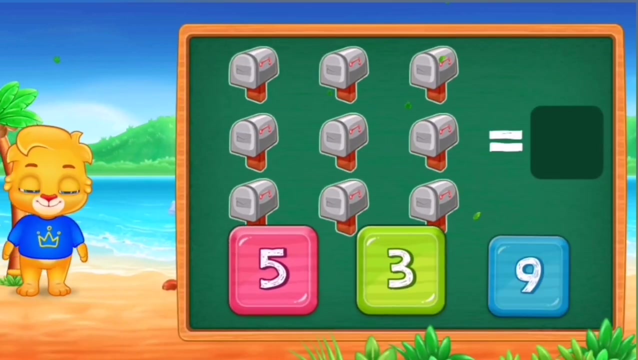 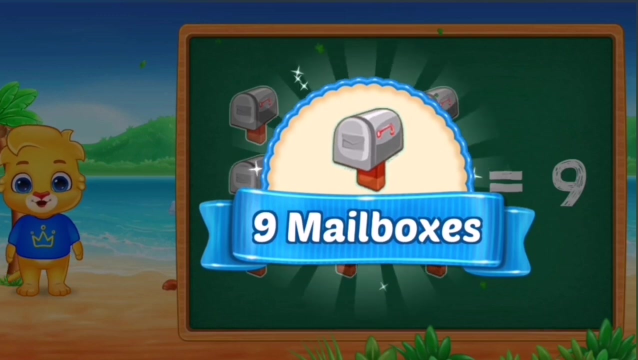 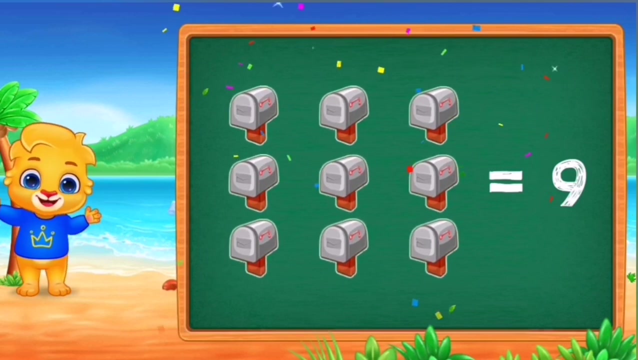 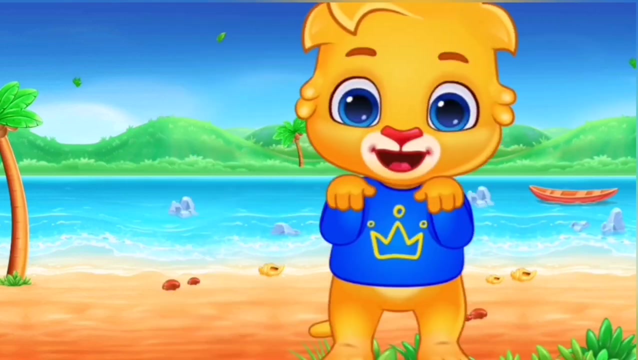 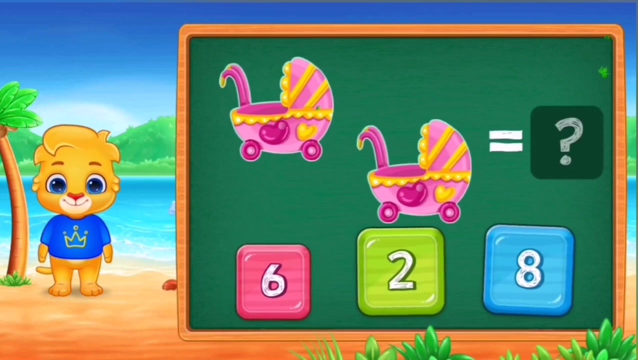 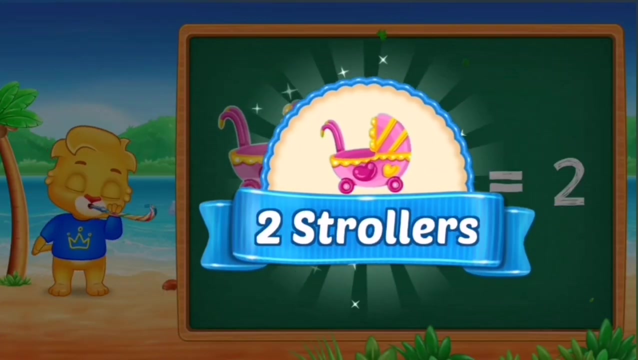 Hi, I'm Lucas. Learn to count. Ten, Ten guitars, Nailboxes, Nine, Nine nailboxes. Let's have some fun. Jump, jump, jump, Jump, jump jump. Strollers. Two, Two strollers. 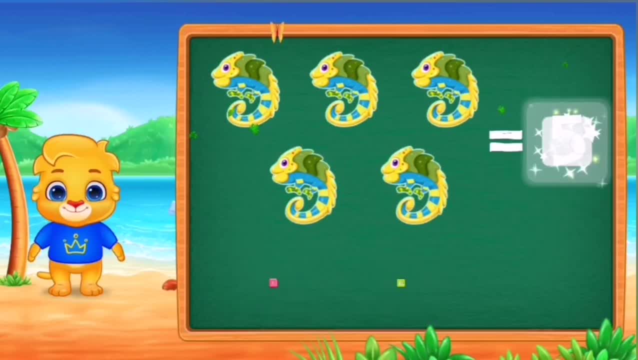 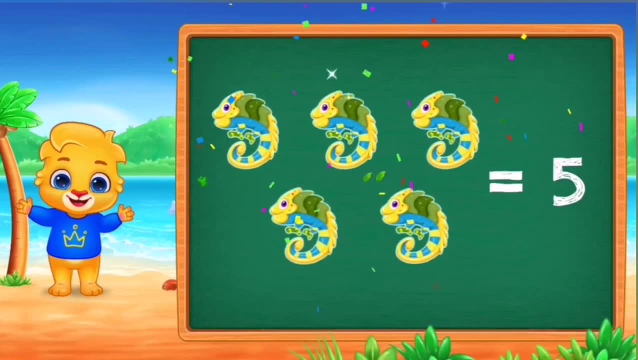 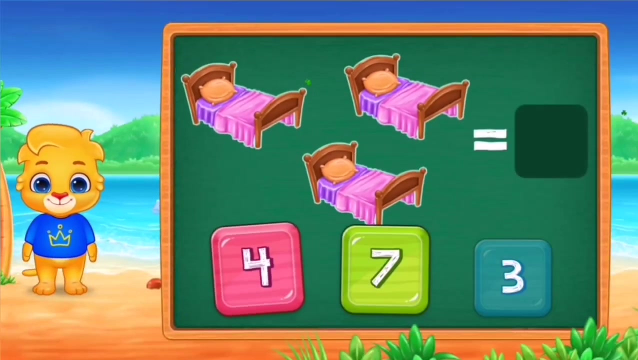 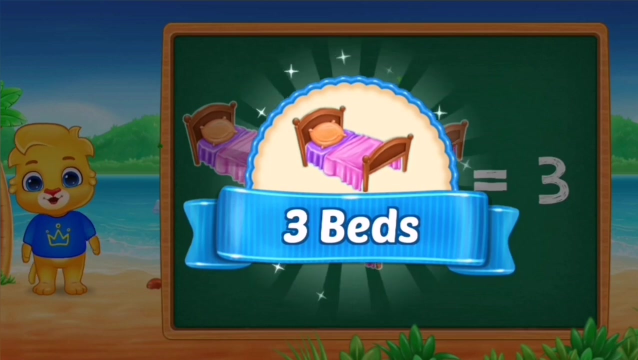 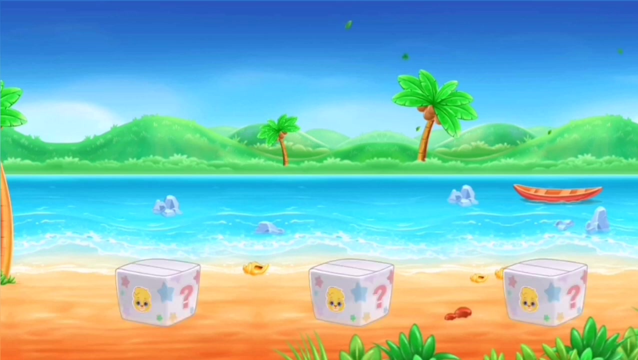 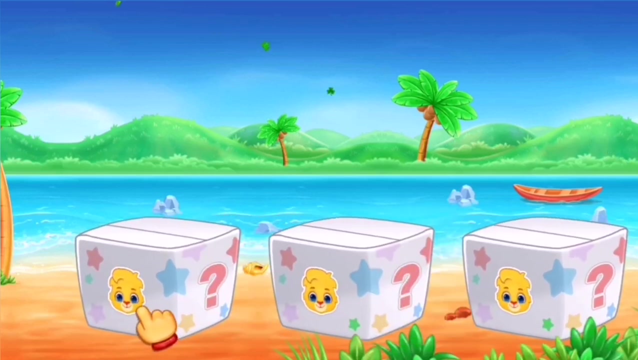 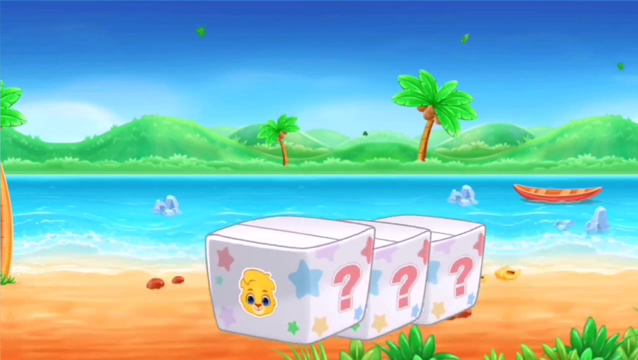 Chameleons: Five, Five chameleons- Good job. Beds: Three, Three beds. I'm hidden in the box. Can you find me? I'm got aBob's. Look, I've found pretty much everything that makes me smile. 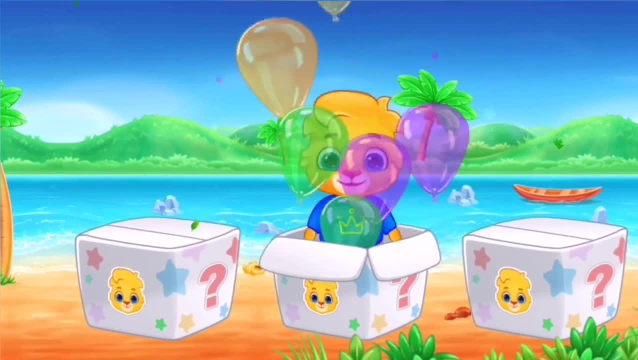 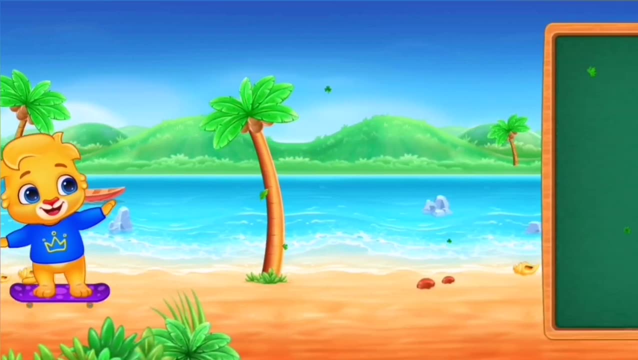 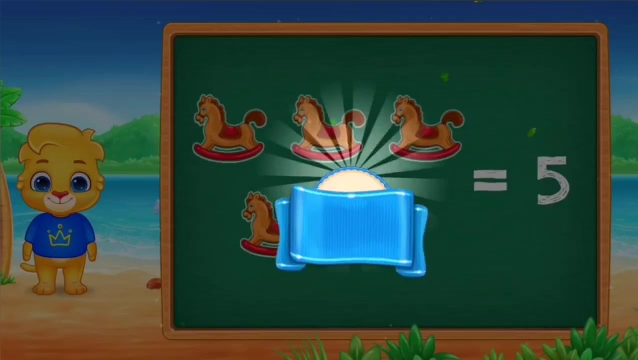 I'm Mrs Newlyweds. Merry Christmas D& Yeah Cos 멤� satisfactorily Anybody have made some simulations. Now that you've wasted your money, let me tell you what you can do. How. How to standing in lines. 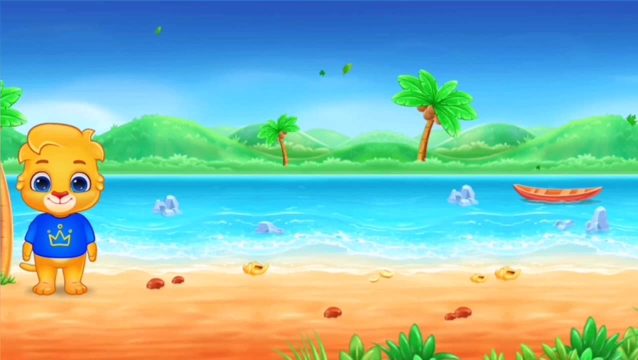 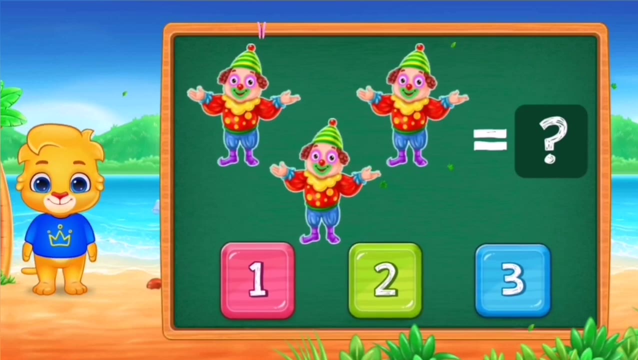 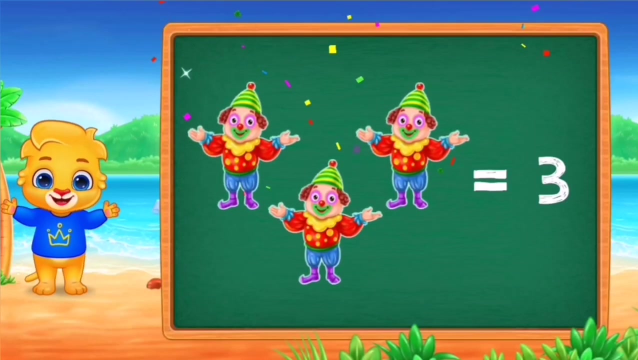 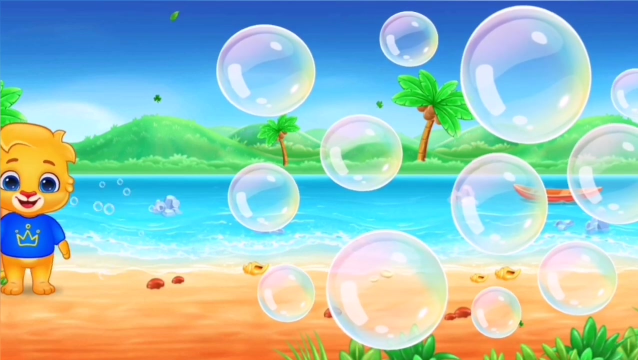 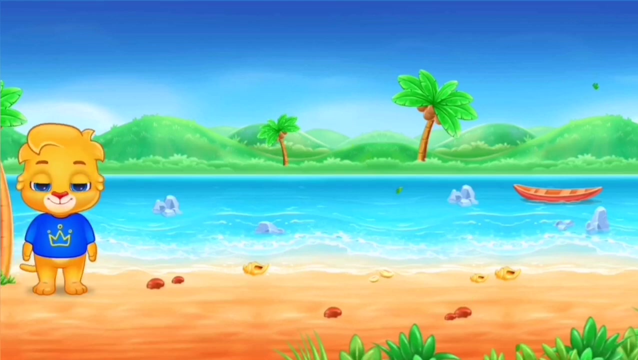 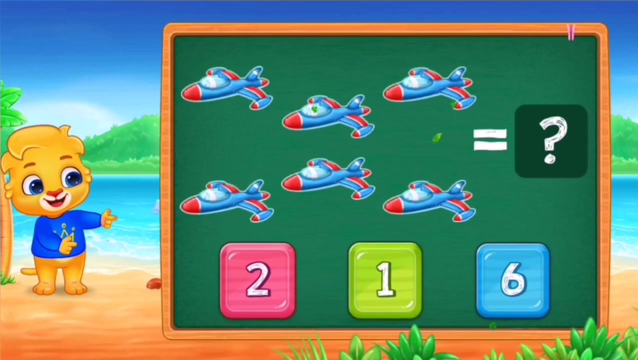 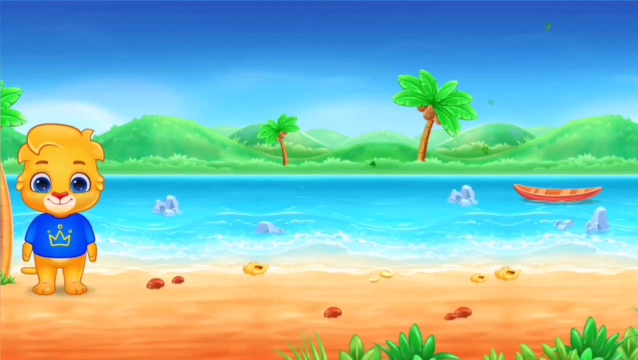 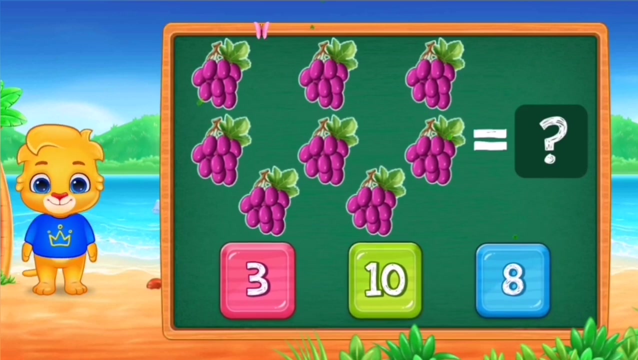 I'm a face mask. This is my new move. Jokers Three, Three, jokers, Wow, Who's ready to pop them with me? Good job. Airplanes Six, Six airplanes. Grapes Eight, Eight, grapes. 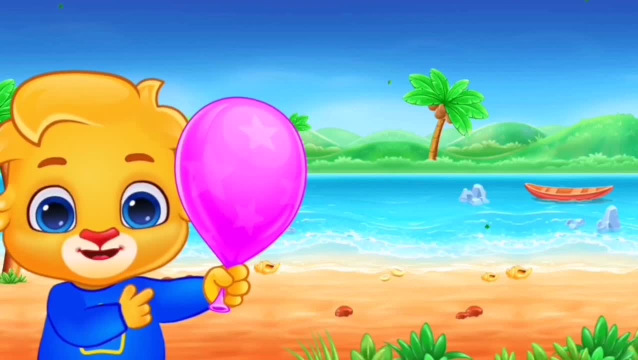 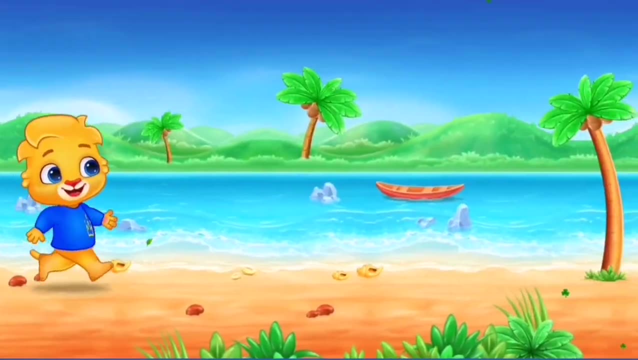 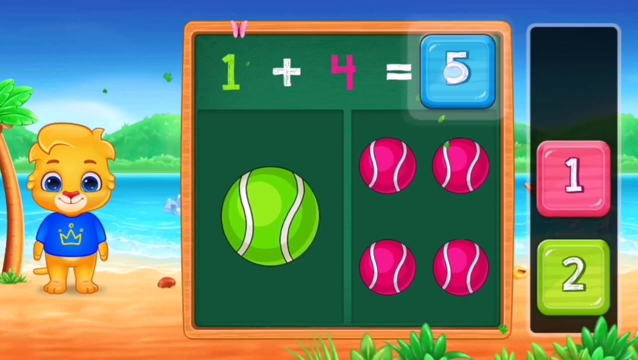 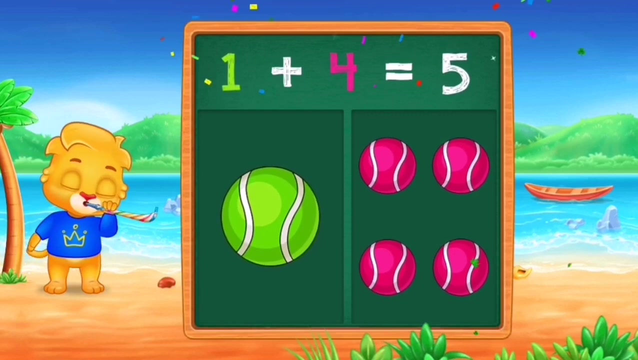 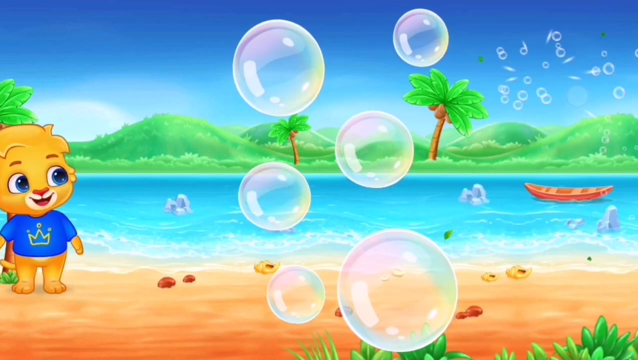 Let's have some fun. Release this balloon. Let's have a balloon on the count of three: One, Two, Three Balls Five. One Plus Four Equals Five. Wow, Who's ready to pop them with me? 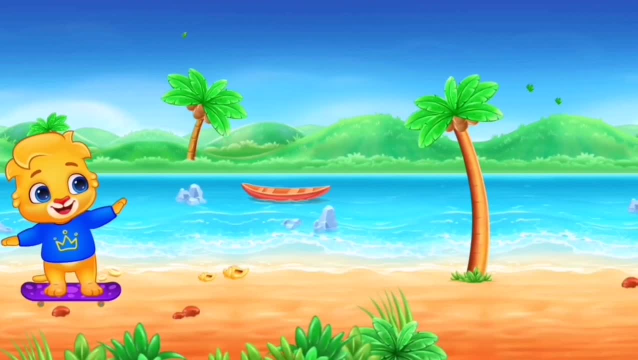 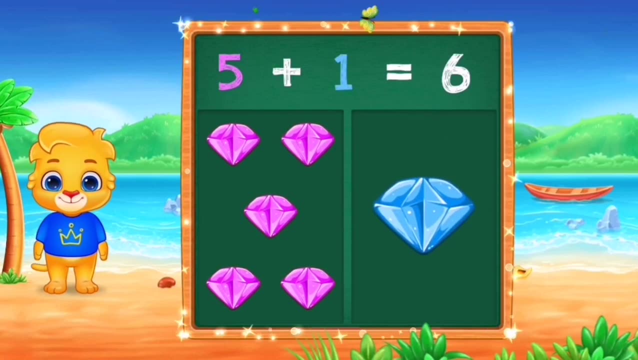 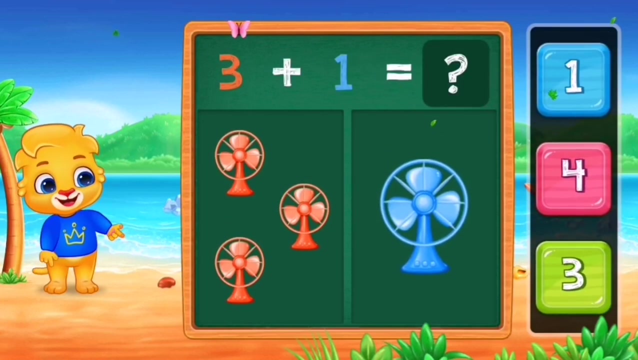 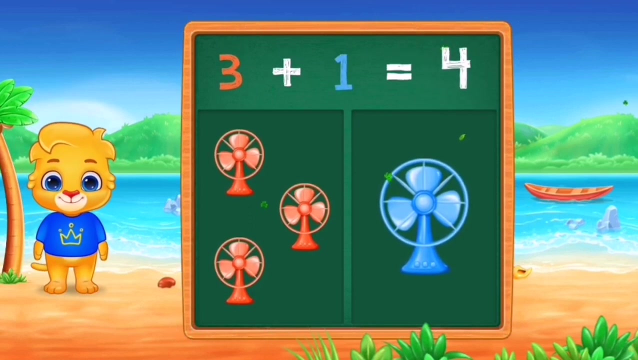 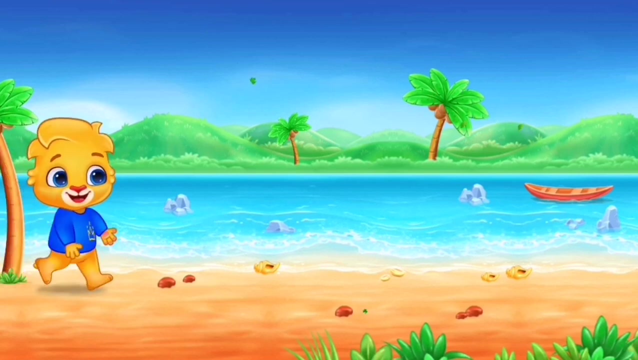 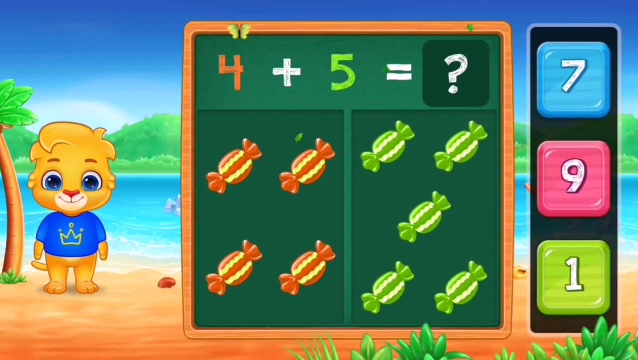 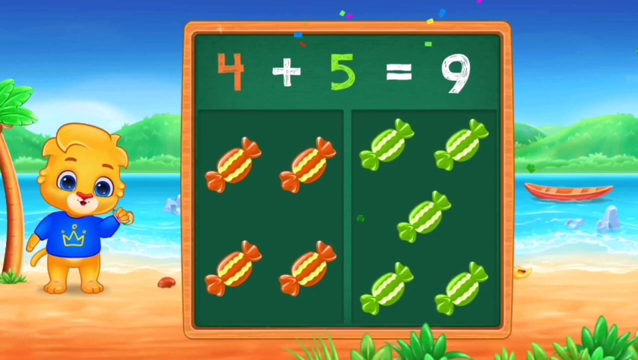 Well done, Diamonds. Six Five Plus One Equals Six. Pan Four Hooray Three Plus One Equals Four. Chocolate Nine Four Plus Five Equals Nine Four. 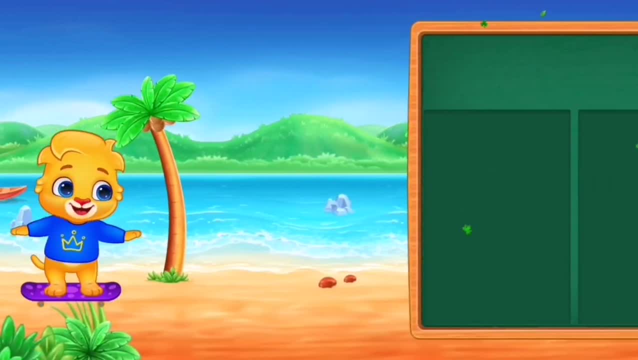 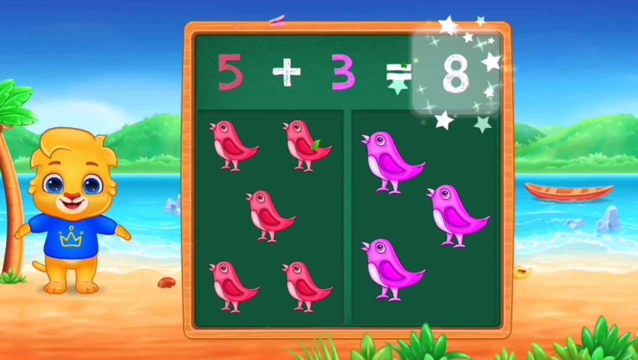 Plus Five Equals Nine. Four Plus Five Equals Nine. Six Birds: Eight Woohoo Five Plus Three Equals Eight Ice creams. Two Woohoo One Plus. 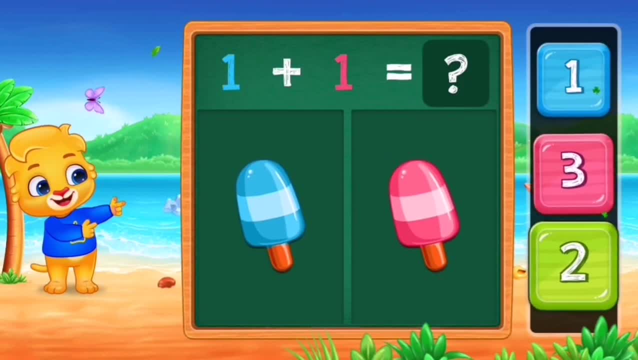 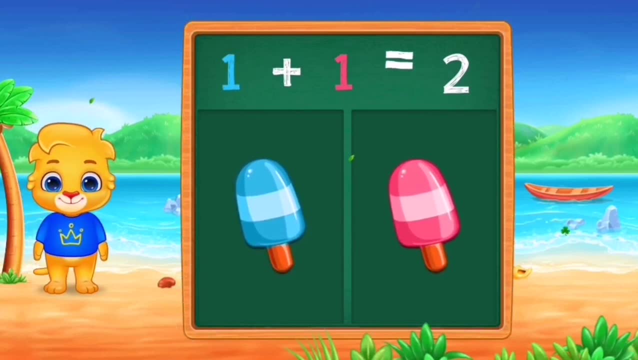 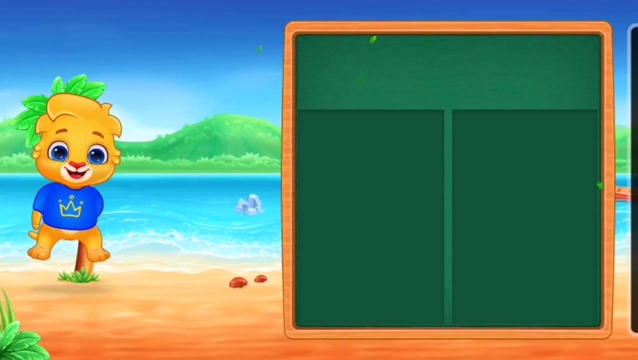 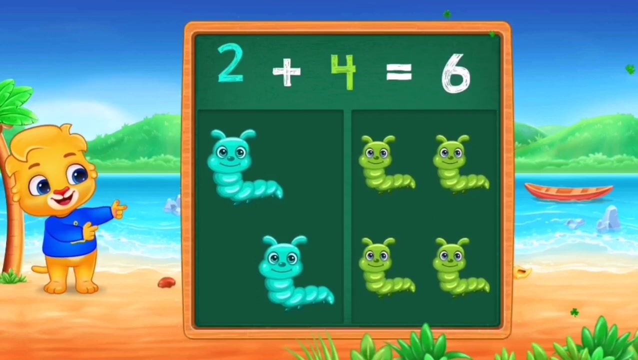 One Equals Two Ice cream, Two Woohoo. One Plus One Equals Two. Two Ice cream, Two One Ice cream. Two Plus Four Equals Six Six Six. 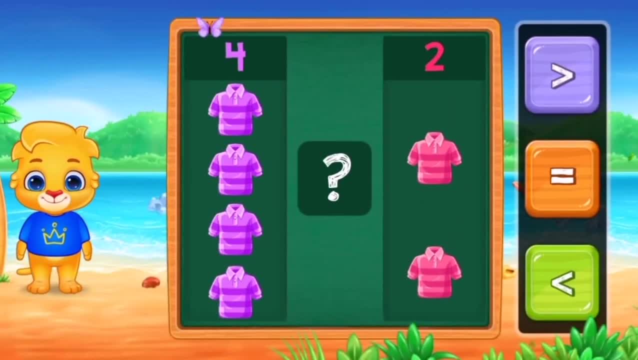 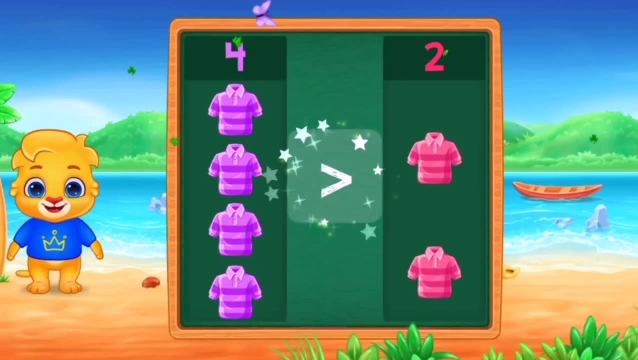 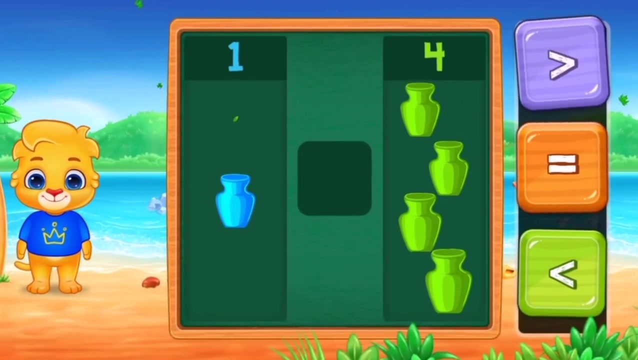 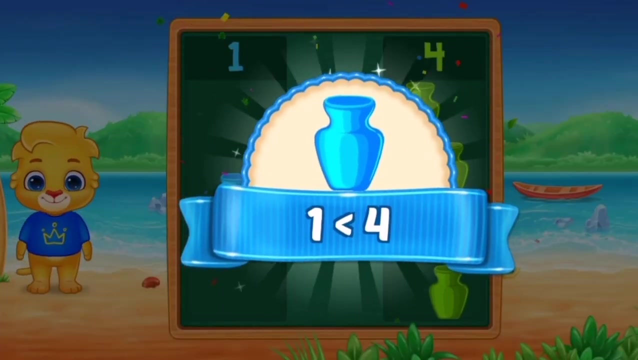 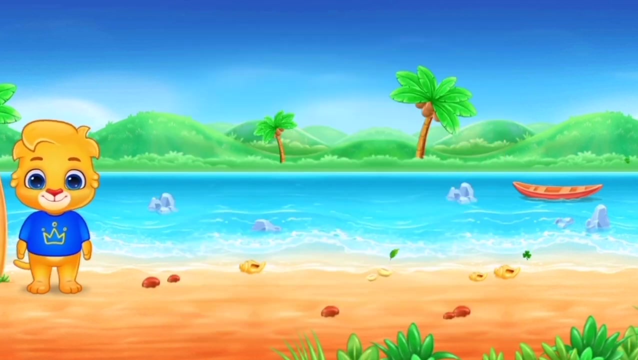 The numbers Two Plus Four Equals Six, Six The numbers Woohoo. Two. Four is greater than two. Hooray Pots Less than One is less than four. Hooray, Let's have some fun. 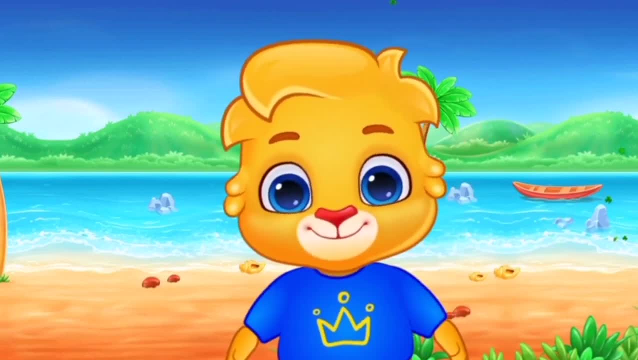 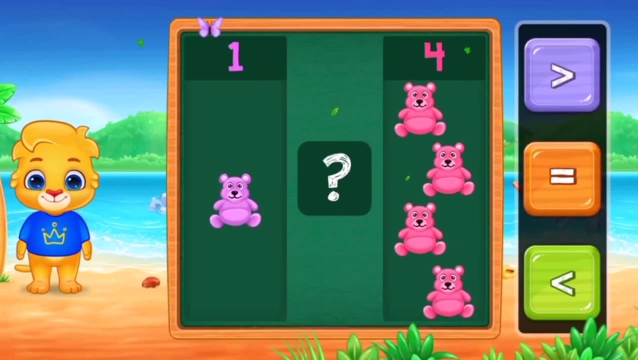 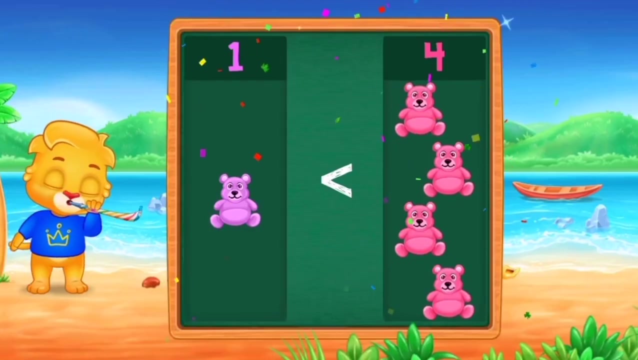 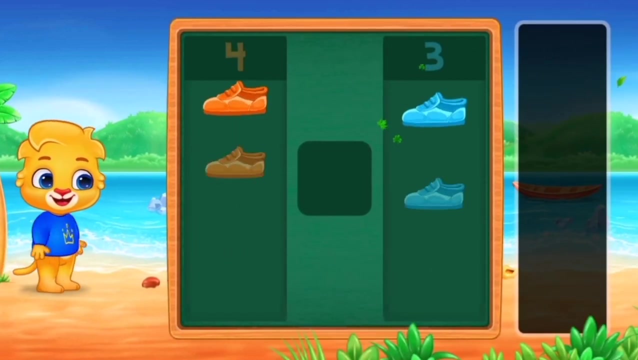 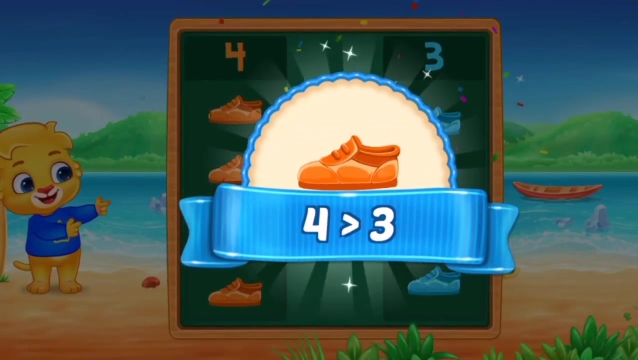 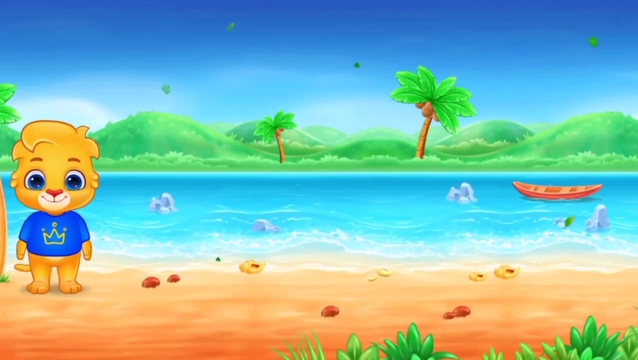 Jump, jump, jump, Jump, jump jump. Teddy bears: Less than One is less than four. Hooray, Hooray. Shoes. Greater than Four is greater than three. Hooray, Good job. I'm Lucas. 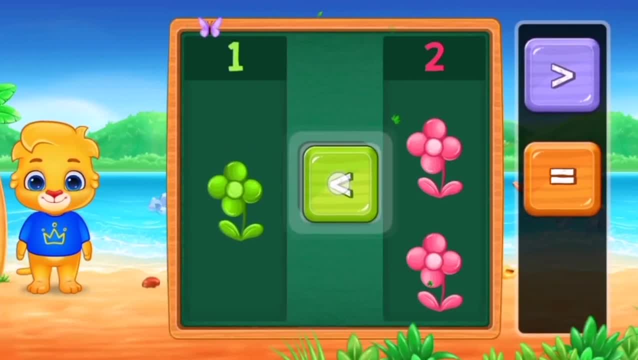 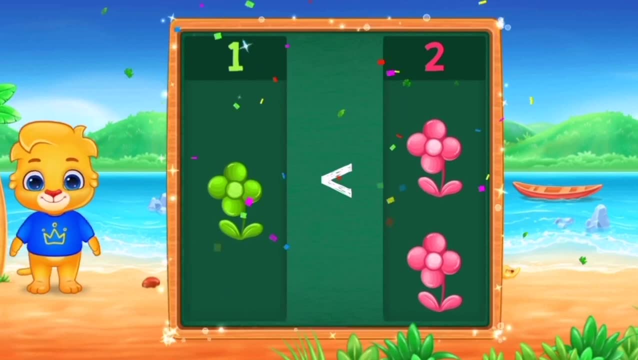 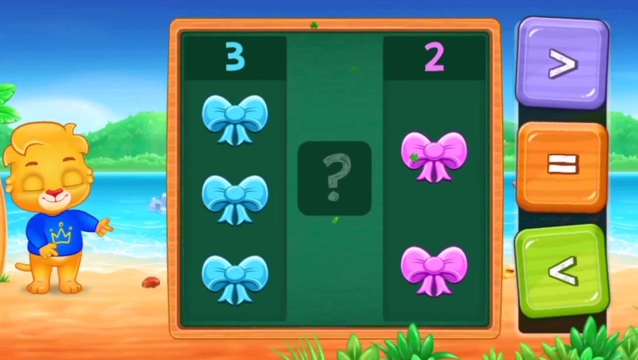 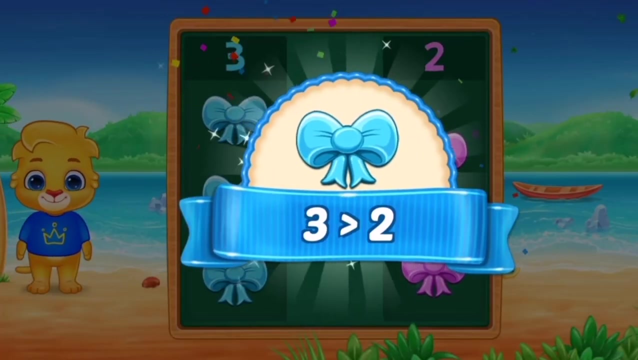 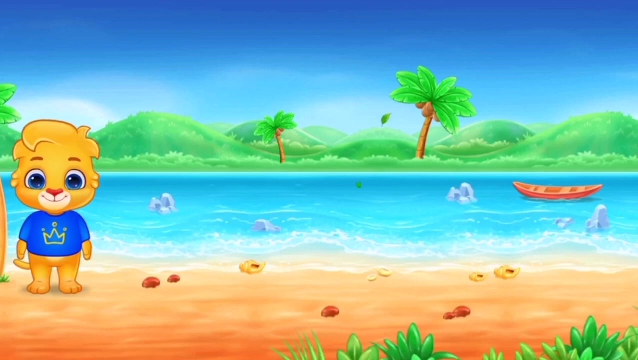 Flowers Less than Hooray. One Is less than Less than Two. Hooray Bo Greater than Three. Three is didn't seem too far off. Three is greater than two. Hooray, I'm hidden in the box.